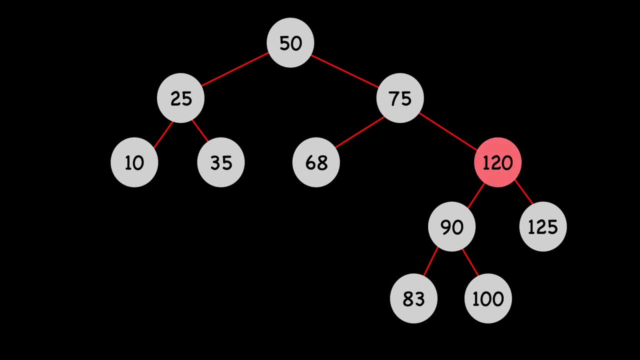 Lastly, let's delete node 120.. This node has both a left and a right child, so we need to find its in-order successor. That is, the node in the tree with the smallest value that is greater than 120.. You can see that this is 125.. 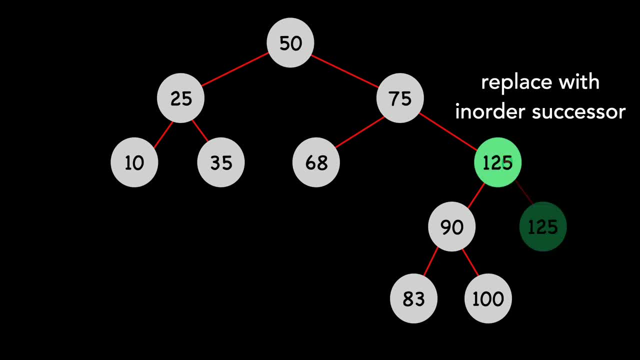 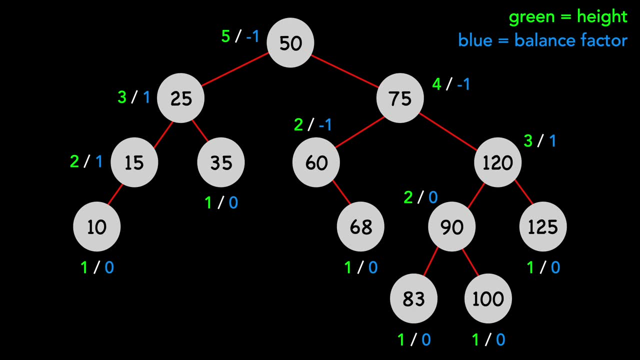 So we move 125 to the left child. We move 125 in the place of 120.. Now let's go back to our original tree, this time filling in height and balance factor, and I'll show you a few examples of rebalancing after removing nodes. 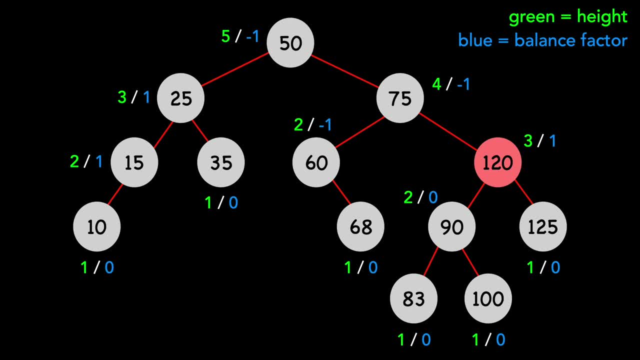 Let's delete 120 again. We move 125 in its place. It now has a height of 3 and a balance factor of 2. Which we know breaks our AVL tree property. So we need to perform a fix. Here are the four types of fixes, which are very similar to insertion. 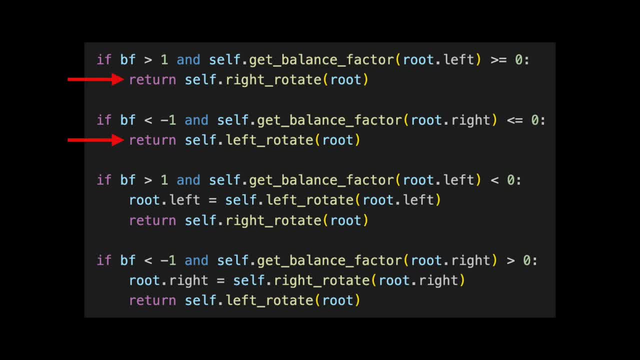 We see that we can perform single or double rotations. We analyze the balance factor of the node and the balance factor of its left or right child to determine if the tree is left or right heavy. I'll draw in the subtree of interest and let's run through the logic. 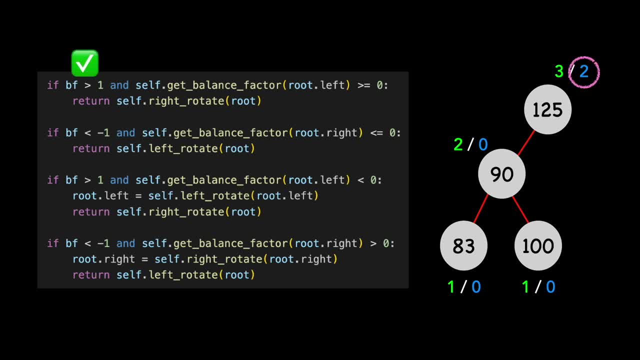 Our balance factor is 2, so this first condition is met. The balance factor of its left child is 0, so both conditions in the first if block are true, We need to perform a right rotation Back to the full tree. I'll demonstrate a right rotation on node 125.. 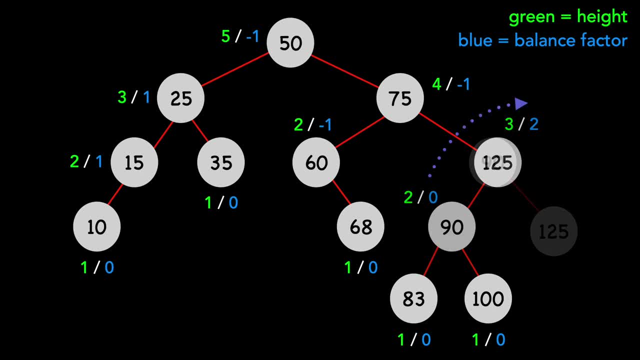 We're back to a balanced AVL tree. Let's do one more example, this time deleting 10.. It's a leaf, so we don't need to replace any nodes, Just remove node 10.. The height of 15 updates to 1..